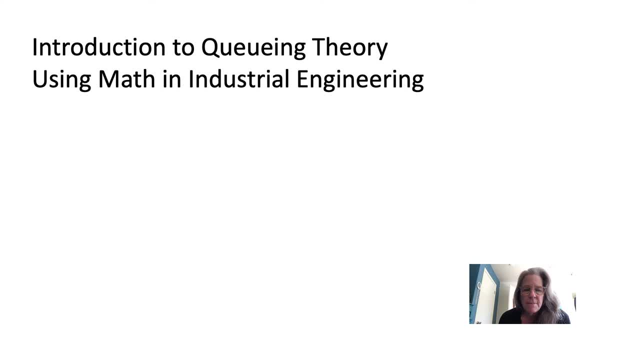 theory is in the simplest form and the simplest aspects of it. I'm also going to then work through an example and show how it might be used in analysis. So queuing theory is the concept of there's items, people or parts or anything that needs to be processed by a server who 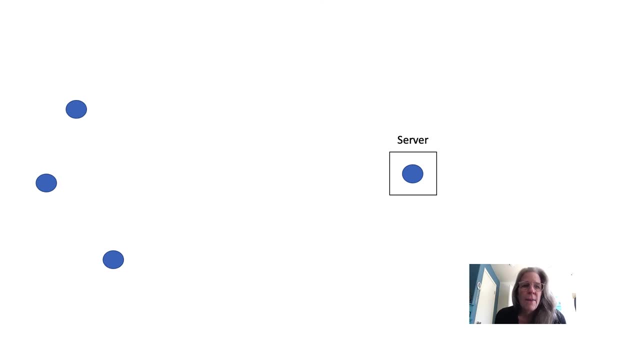 does some work that takes some time on the items or with the people. So the way we usually conceptualize this is these: the three dots on the left is what I'm saying- are the item number 1 and item number 2.. They're the items that we take out of the collection. 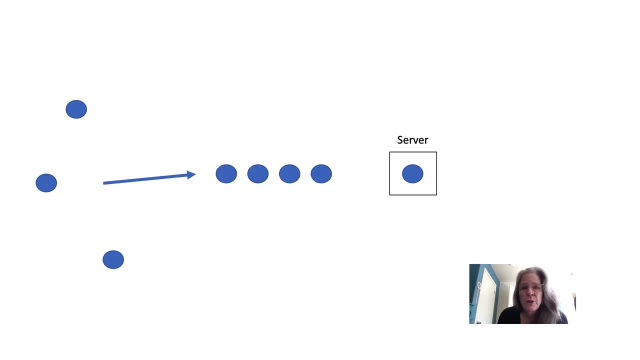 that need to be served. they start to move towards the server and form a line and then, as that, as the server is available, um the process, one person in the line or one item in the line is served by the server and then exits the system. so we call this line a queue and that's what we call. 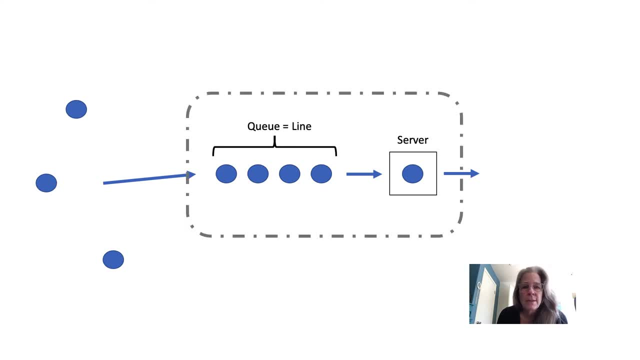 queuing theory and then the whole system is we define as the line and the server, so we don't include the items that are traveling to the system. so we draw the system this way. one of the important things about queuing theory is to really define the type of queue you can imagine. 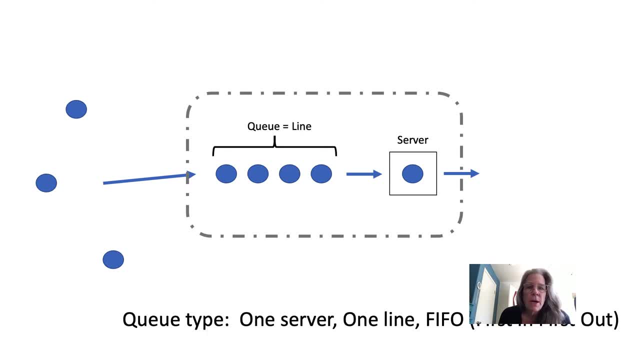 there's all kinds of different types of queue. this particular type of queue is a one server, one line, first in, first out. so that means the first items to get in the line are the next ones that are going to be processed. so we travel through the line this way. 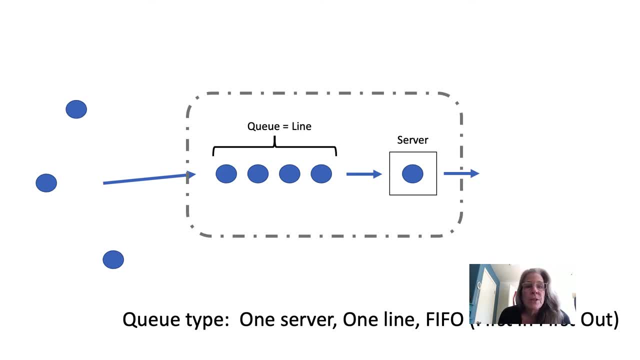 now there's all these different types of queues that we're going to talk about in this video, all kinds of other types of configurations for queuing theory. there could be multiple server one line first in, first out. there could be multiple server one line last in, first out. 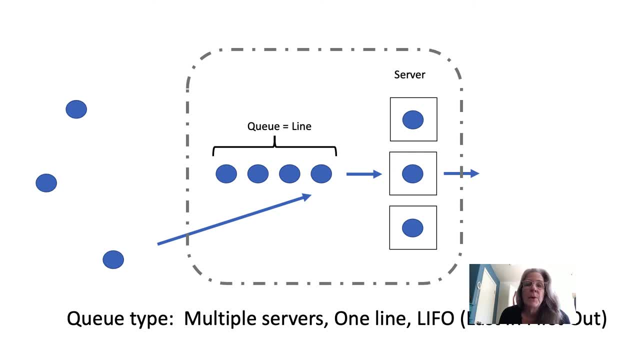 so instead of going to the end of the line the, the next item goes to the front of the line. now, all of those indicate a different kinds of calculation, but the calculations i'm going to talk about right now are a one, one server, one line. last in first out: type queue. 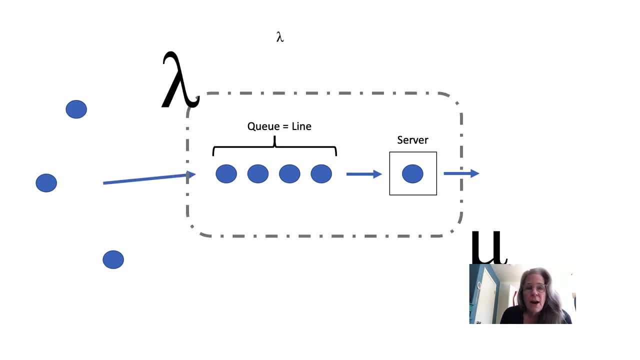 and in this particular orientation, what we do is we define a lamba and a mu, which is: the lamba is the arrival rates and the arrival rates. what we say is: lamba is an expected time of a arrival, arrival per hour and that, but these vary. there's a distribution associated with it and we define 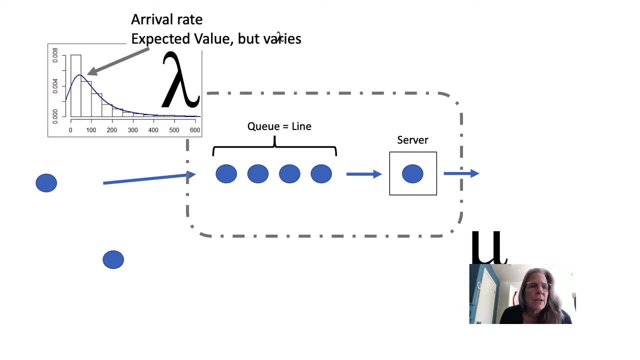 the distribution as exponential. so that looks sort of like this, where we have a lamba, that is the, the expected value, but it's distributed over time. mu is an indication of service rate and that's there's also an expected value, and that varies over time. so we can think about these things as distributions. 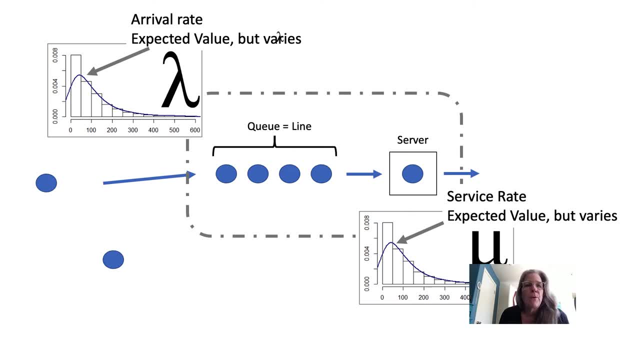 like sometimes, um you, there's two people that arrive together and then sometimes there's like 10 minutes until the next person arrives and then in the service rate, sometimes the service takes 10 seconds and sometimes it takes three minutes. so the service takes three minutes, sometimes it takes. 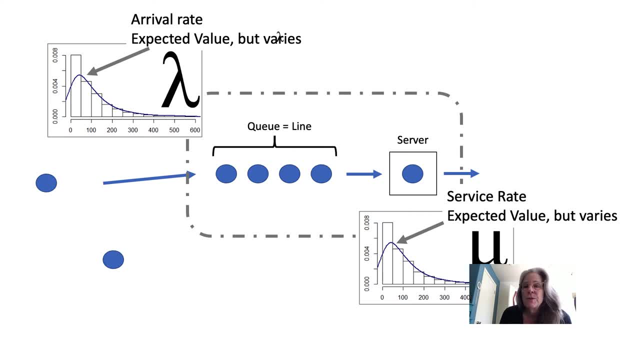 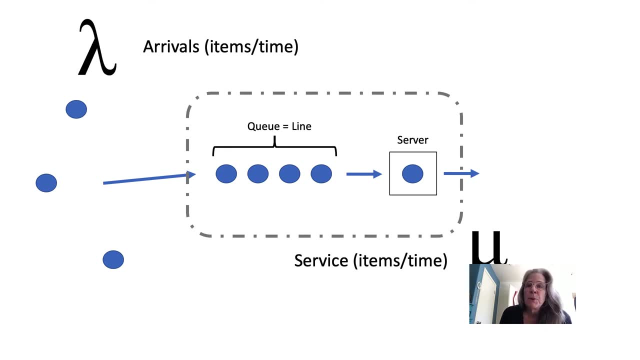 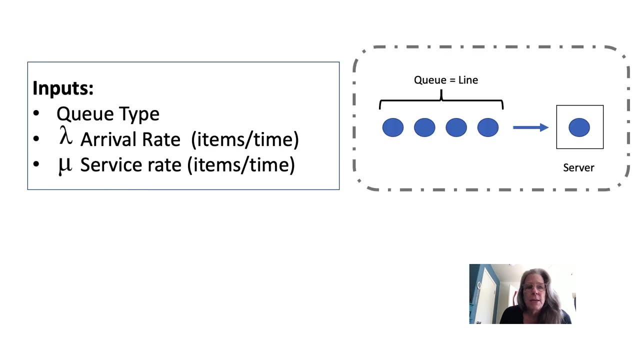 three minutes. so there's a variety as a distribution of the service rate. so what we do is we have these lamba and mu, where the arrivals are expressed in items per unit time and the service is also expressed in items per unit time. so the input in a queuing system is the queuing. 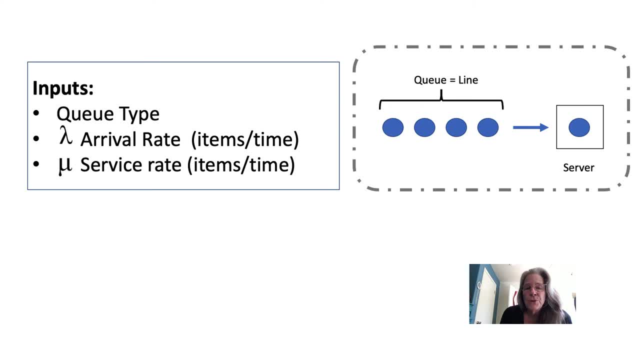 type, which in this case we have a one line, one server, first in, first out, and then we also have an arrival rate and we have a service rate, and that's kind of all we need, and then through some um, really kind of neat math that you will understand if you actually study this in depth, 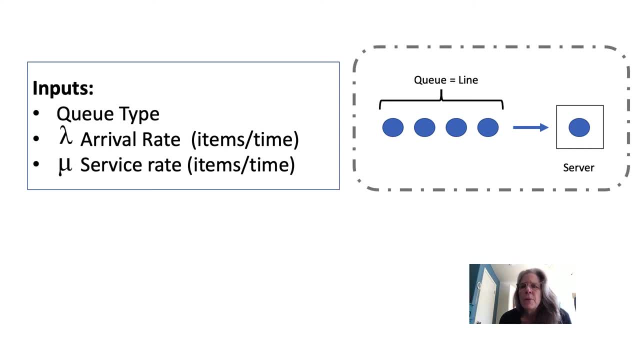 we can actually describe things about the system in pretty simple equations and examples of the ways that we can describe the system- and there's actually a lot of ways to describe the system, but examples are: we can talk about the capacity utilization. we can talk about the number of people. 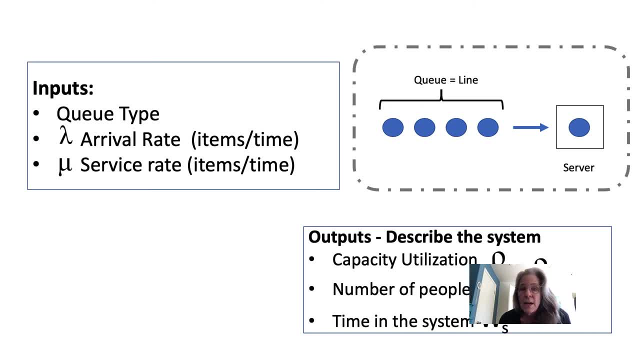 in the system. we can talk about the time that, that people or items. we can talk about the time in the system. so simple equations like the capacity utilization is lamba over mu? pretty simple equation: the number of people or number of items in the system is a row, or the capacity utilization. 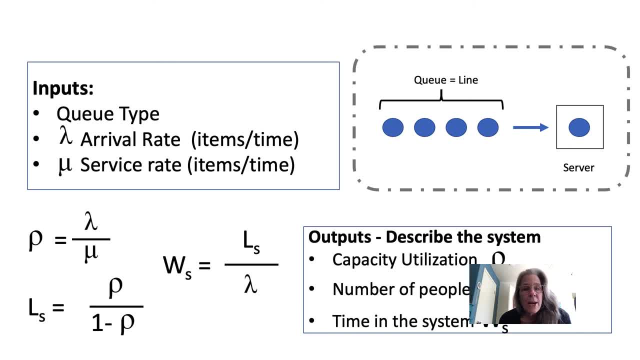 divided by one minus row, and then the um waiting time in the system is the, the number of people in the system divided by lamba. so we have these pretty simple equations that are actually complex to derive, but they're based on distribution of arrival rates, and i'm 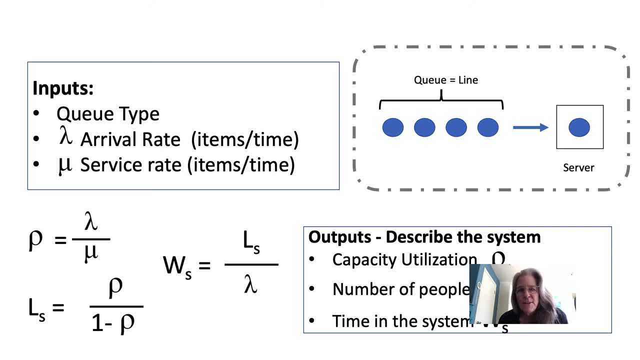 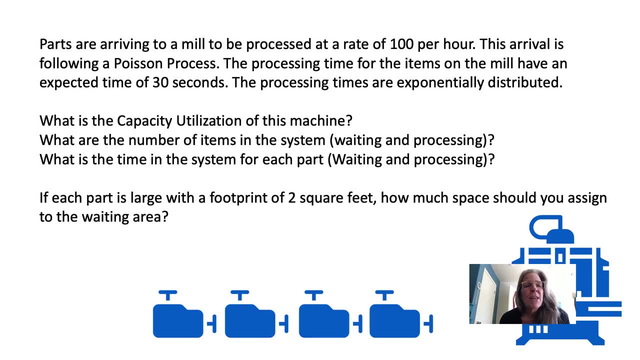 going to go through a really quick example of this. well, not, maybe not maybe really quick. i'm going to go through an example. so in this example it's um. parts are being arriving to a mill, a milling machine, and they're going to be processed, and they arrive at a rate of 100 per hour. 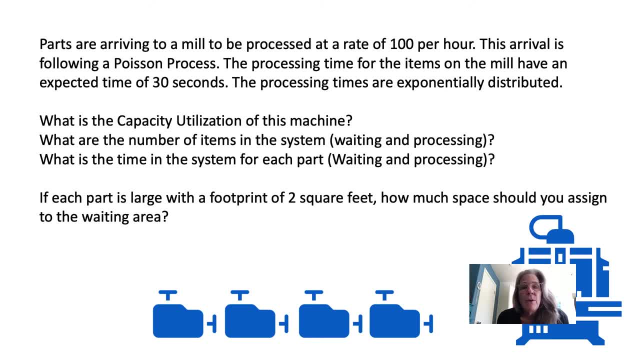 this arrival follows a poisson process and the processing time for the items on the mill have an exp expected um rate of 100 per hour. so the processing time for the items on the mill is about um time of processing of 30 seconds and the processing times are exponentially distributed. 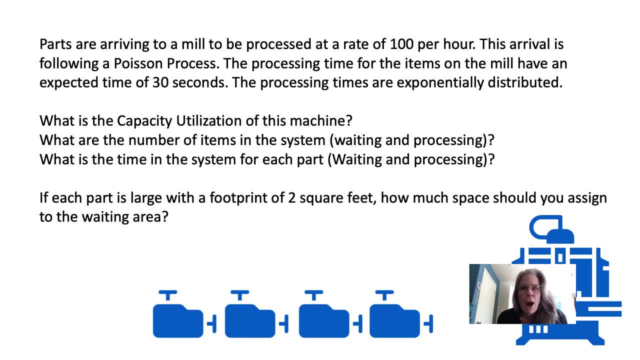 so the first question is: what's the capacity utilization of the machine, that means how much of the time the machine is being used. and then what is? what are the number of items in the system, both waiting and processing, and what is the time in the system for each part, like, how long are the? 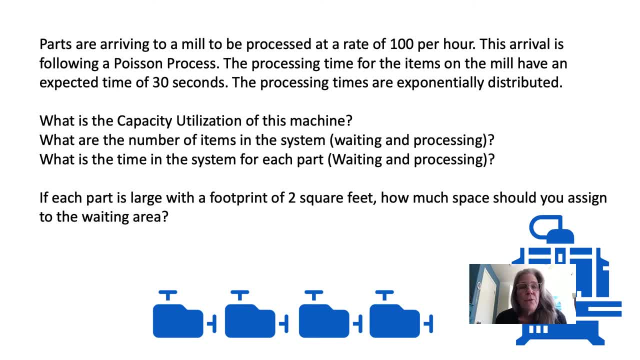 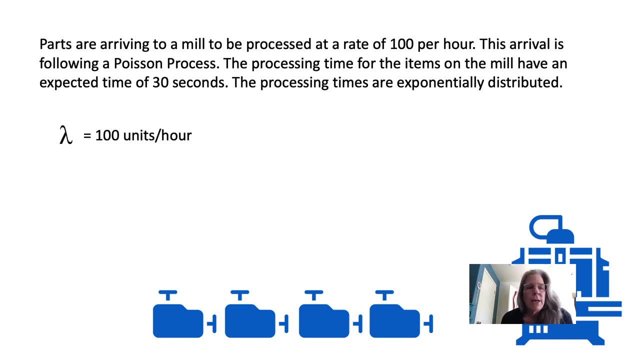 items going to be waiting there, and if each part is large with a footprint of two square feet, how much space should you assign to the waiting area? so these are some of the questions we can get from this simple um queuing problem. so in this queuing problem we initially can just establish lamba, which is the arrival rate, as 100 units per. 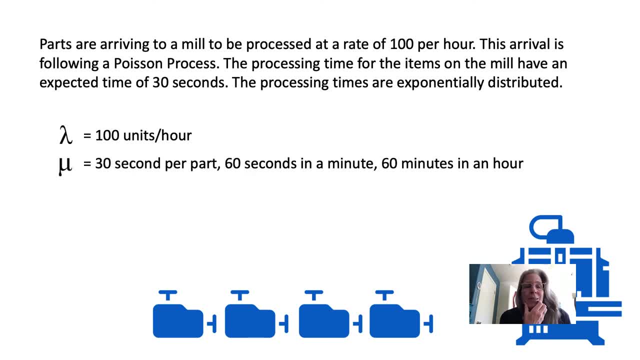 hour. um, the mu is a little bit harder, because what we see is it takes 30 seconds to process the part. that's the service time and we have to make sure that the mu is actually in units per hour and the 30 seconds per part is actually seconds per part, which is not the right unit. 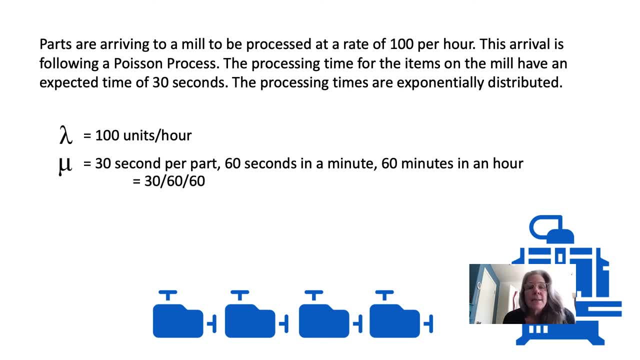 so we have to take into account that there's 60 seconds in a minute and 60 minutes in an hour. so, matt, that means it takes 0.0083 hours to process a unit. but still that's not quite the right units for mu. the right units per mu is one unit per 0.0083 hours, which means 100- 120 units.